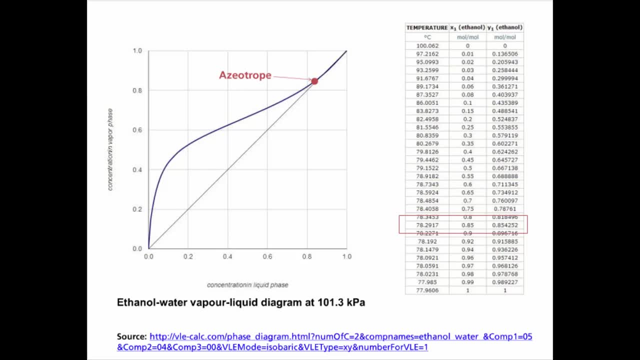 which the composition of the liquid is almost the same as the vapor and touches the XY line, making that the maximum separation that can be achieved using conventional distillation is approximately 85% or more. This means that the solution of pure distillation in azeotropic 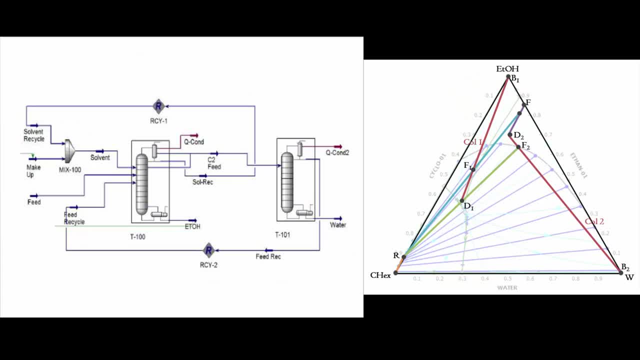 distillation is more or less 85% in mole fraction. The azeotrope can be break using an entrainer. Typically, the data we know when designing an azeotropic distillation system are the flow rate and composition of the ethanol and water fit and the desired composition of the ethanol and water. 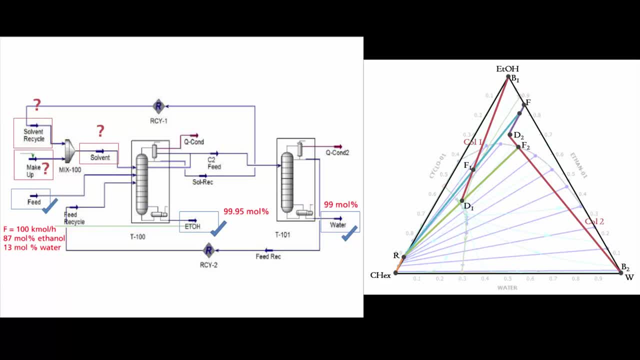 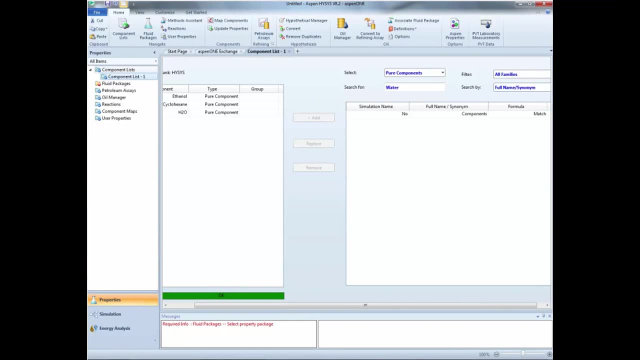 products And we need to find out how much entrainer is needed to achieve the ethanol purity trainer and the ethanol for economical reasons. so these streams are recycled back to the first column. In this video. we assume that you already know how to more or less use Isis, so a number of steps are only specified. First, select: 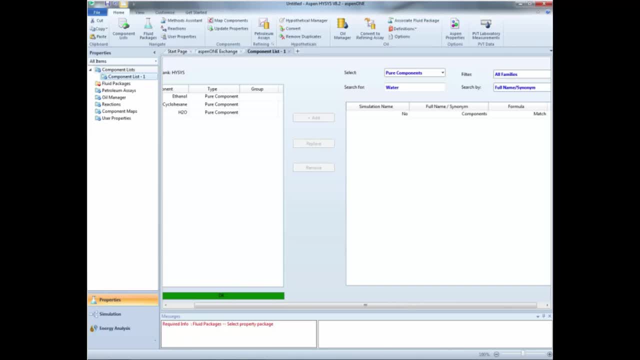 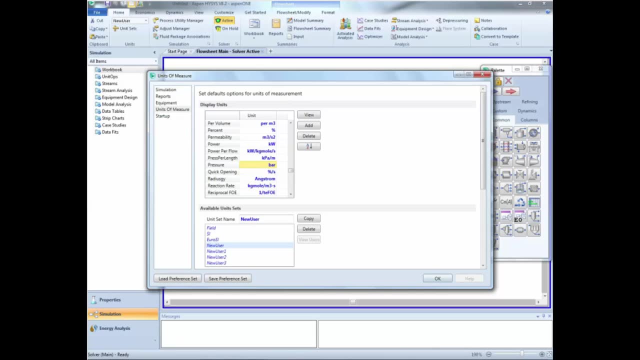 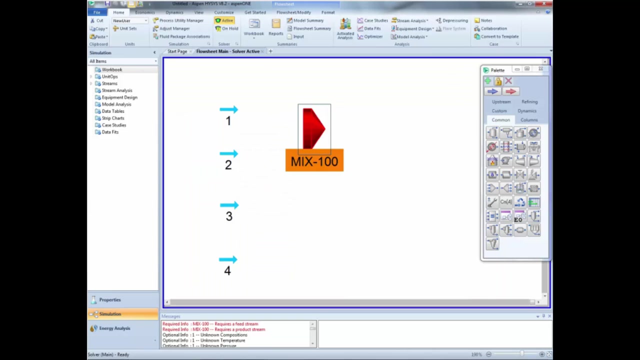 ethanol, cyclohexane and water as components. Now select BrSB as fluid package. Create a new set of SI units in which the pressure is given in bars and not in kilopascals, And in the main flowsheet insert four material streams. 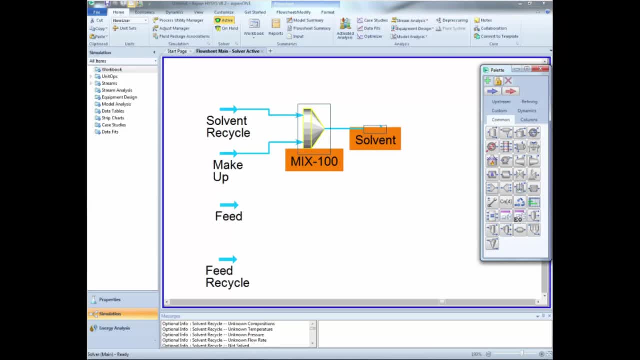 and a mixer Now rename the stream as shown in the video, connect the streams solvent-recycle and makeup to the mixer and create a new stream named solvent, as output of the mixer. We don't really know the inputs of the solvent-recycle and the makeup streams, but we need to define them in order to have a convert. 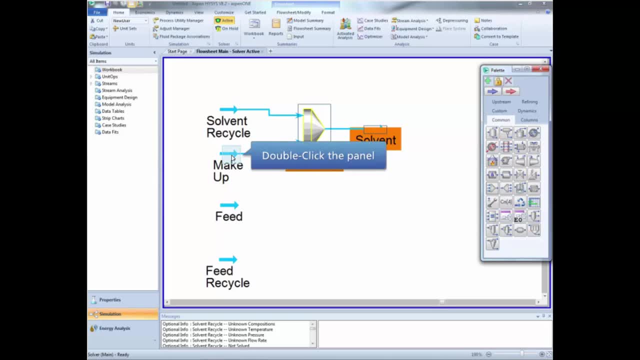 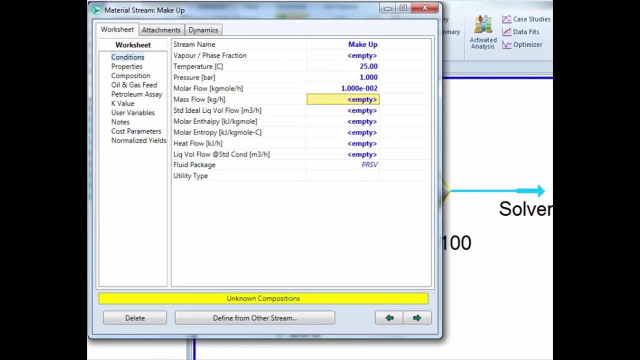 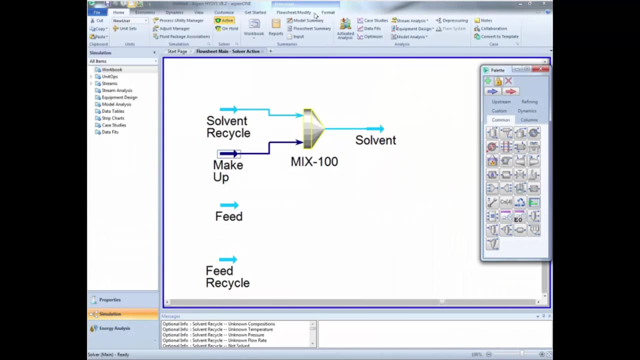 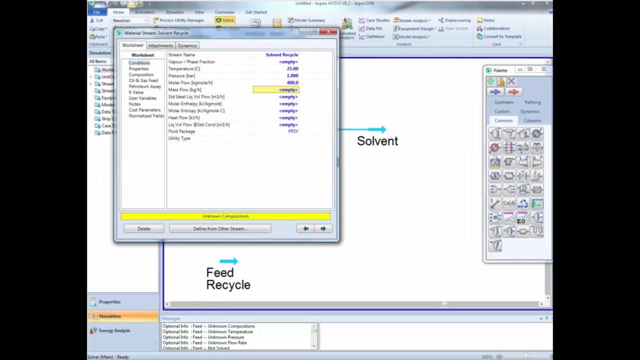 simulation. So double-click on the makeup stream and define the temperature, the pressure and the molar flow as indicated in the video. In the composition tab, define the stream to be pure cyclohexane. Now open the solvent-recycle stream and input the solvent-recycle stream. 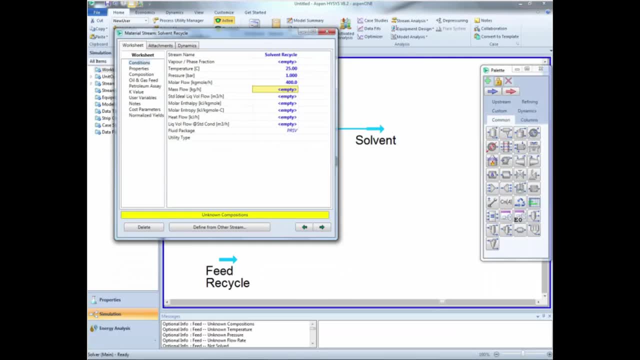 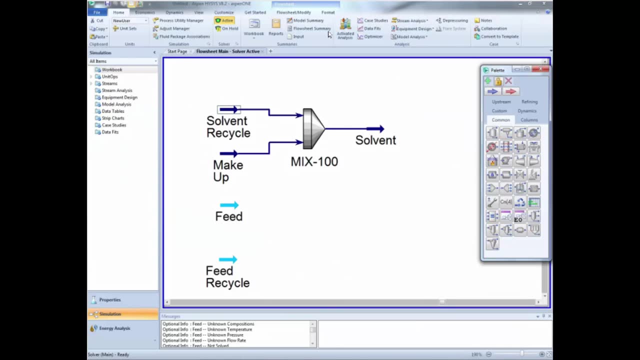 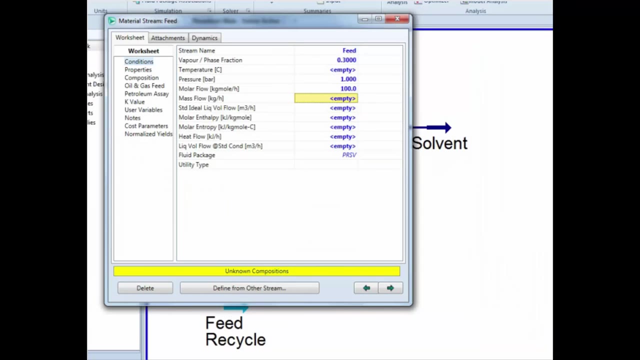 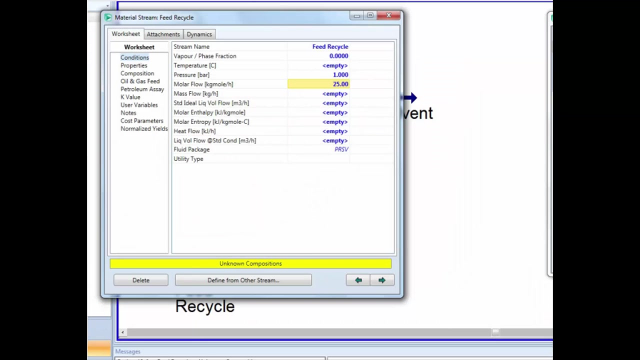 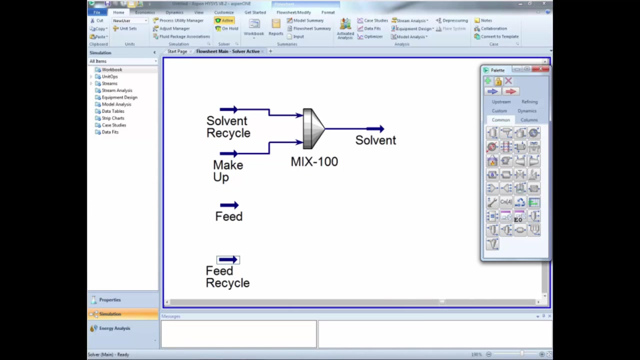 Enter the following values for temperature, pressure and flow rate. Define this mixture to be an equimolar mixture of ethanol and cyclohexane. Now define the feed and the feed-recycle streams as shown in the video. nal crystallization column. the next step is to install a distillation column: click. 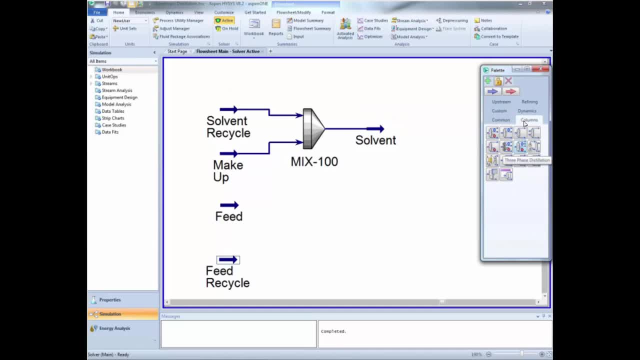 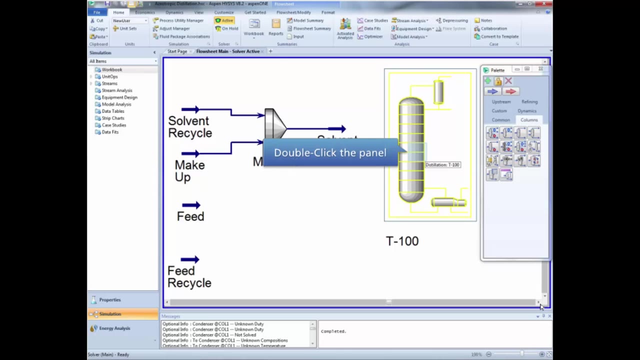 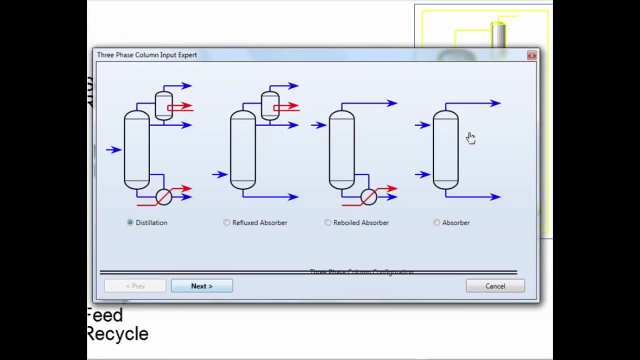 the column label on the palette alliances to the system. tohyunun luis phase distillation column and install it on the flowsheet. Double click the column item to open the columns of flowsheet. In this window we can select the type of separation we want. in this case we want a distillation. 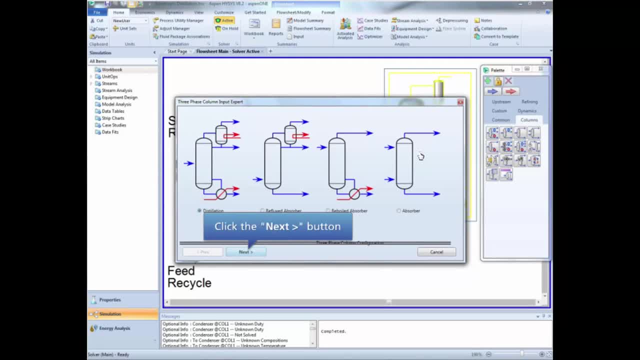 column. that is already selected, so we just simply click next. This new window asks for the number of stages, so we are going to type 62 on the corresponding field and then click next. This window is to select the type of condenser we want. first, type a name for the energy. 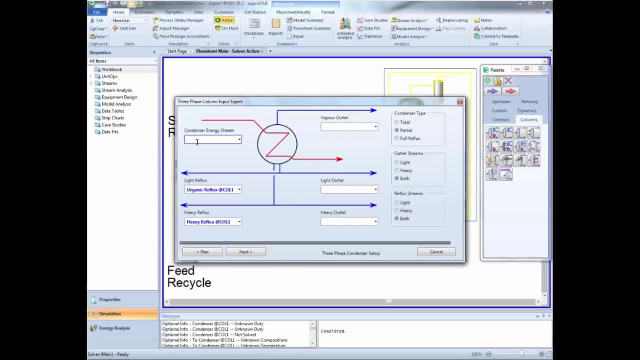 stream. Now select the total condenser and type names for the liquid outlets. Click next when you are done. This new window is to select the condenser specs, but as we don't know any of them, we are just going to move to the next page. 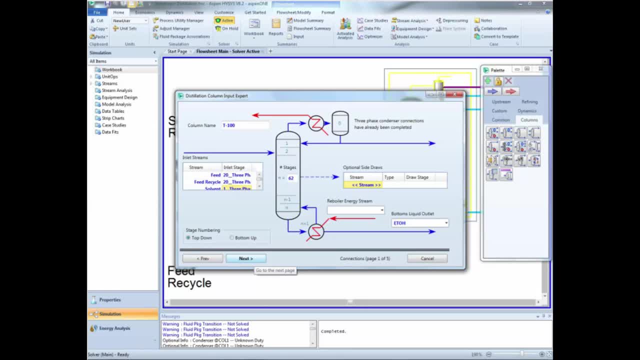 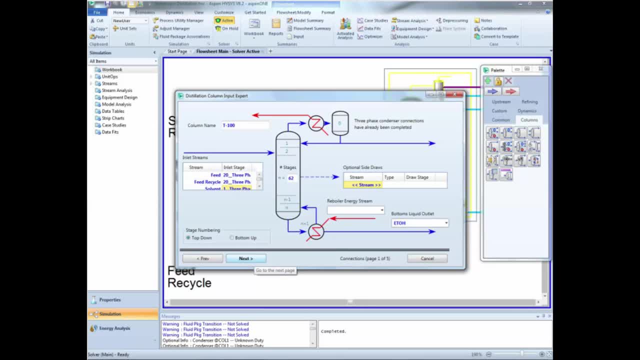 The second will enter the column on the 20th stage and the solvent on the first stage And also give a name for the bottom liquid outlet stream. Once you finish, click next. We only have one choice for the reboiler configuration, so we just simply click next. 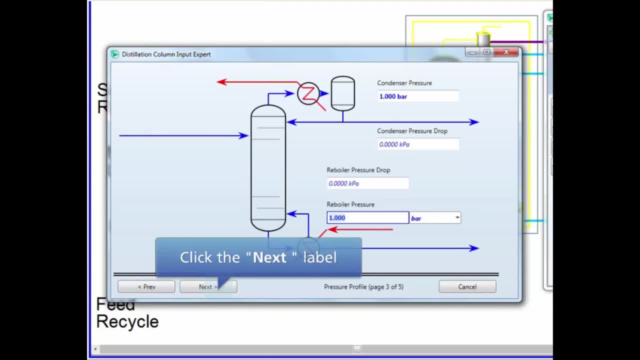 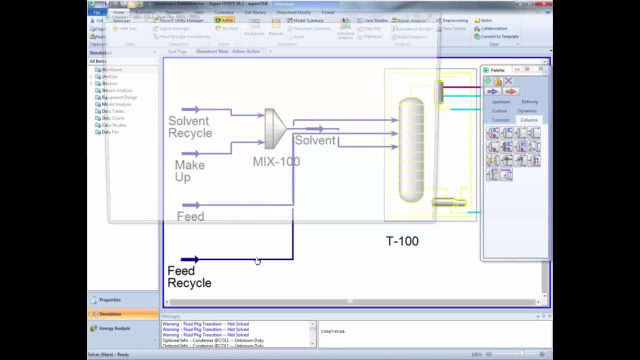 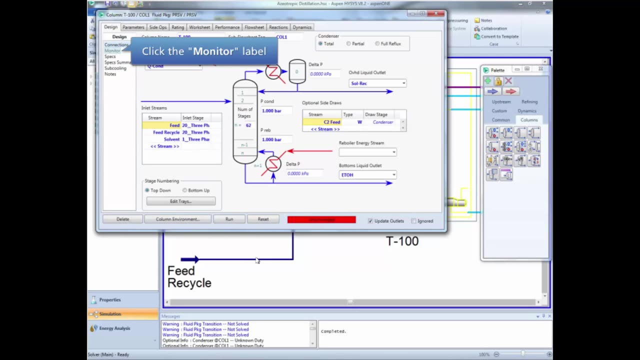 Set the reboiler and condenser pressures to be one bar and then click next. This data is optional, so again, we just click next. Now we need to add some specification to convert the distillation column. so we need to move. 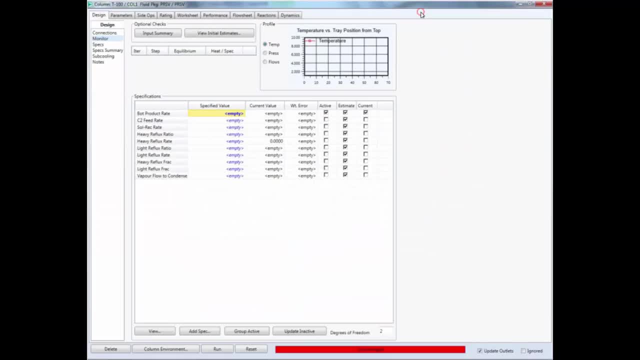 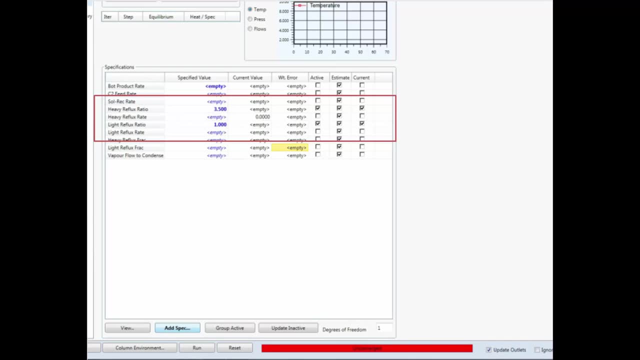 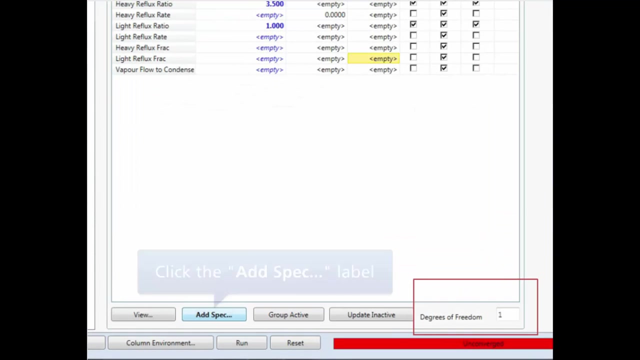 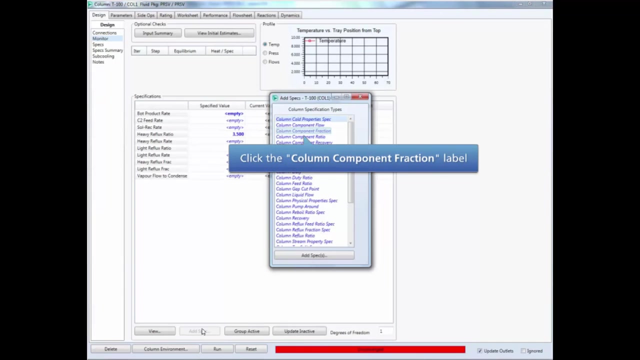 to the monitors page, Now active, only the heavy reflux ratio and the light reflux ratio specification and specify the values as shown in the screen. Note that we still have one degree of freedom, so click the add spec button to add a new specification, Select the component fraction specification and enter the specification for the ethanol. 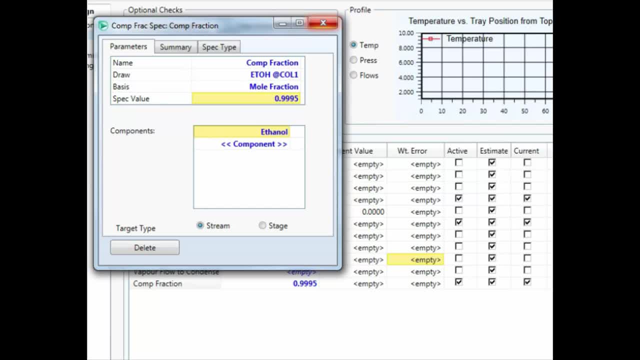 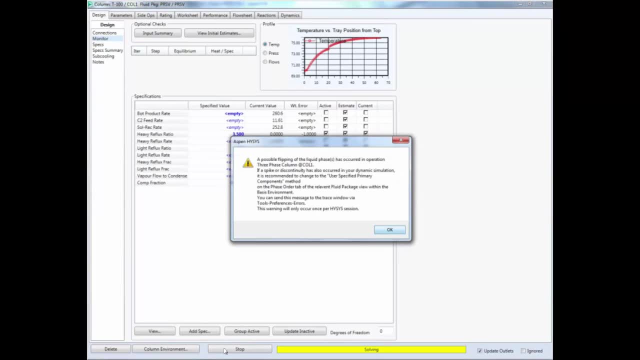 stream at the bottom of the column. Close this window in HISIS. Now click the run button to begin the simulation of the column. If this warning message appears, don't freak out, just click ok. And now we have a convert simulation of the distillation column. 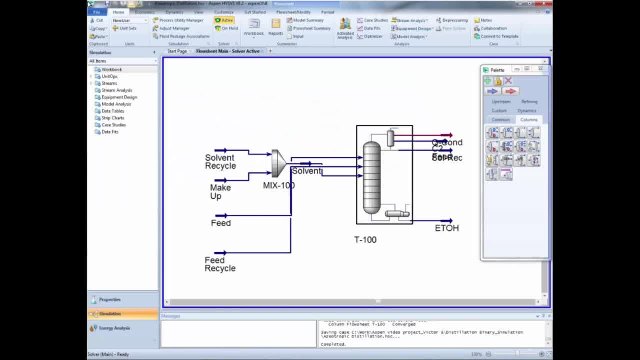 You can close this window now. As you remember, at the beginning of the video it was mentioned that the inputs for the solvent recycle and the makeup streams were unknown, and these values were assumed in order to get a convert simulation. In this section of the video, we are going to learn how to use HISIS to calculate these. 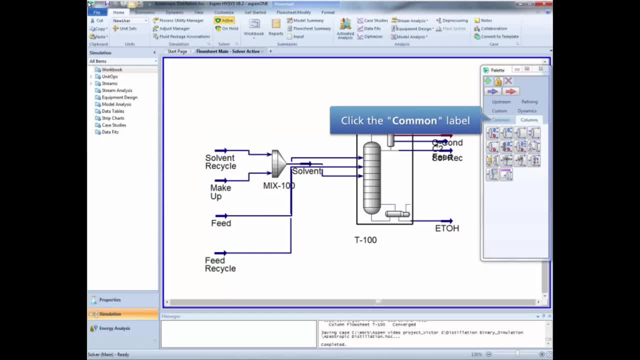 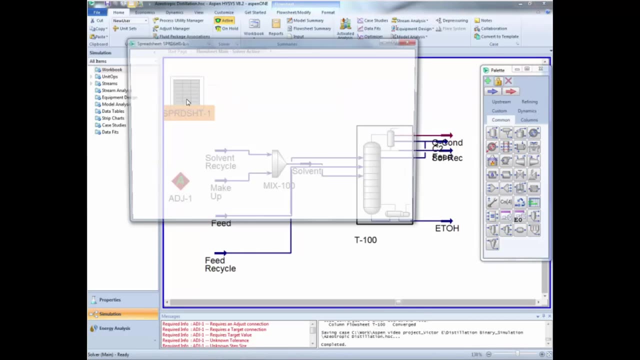 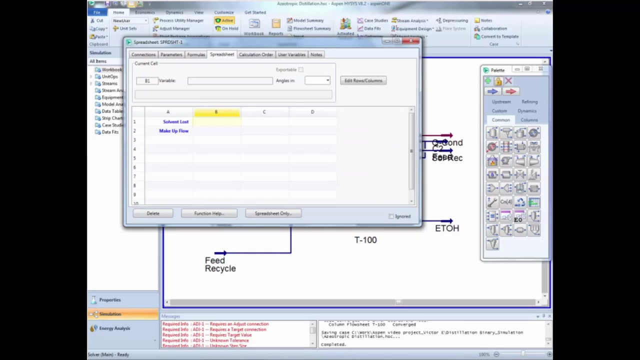 values. First we are going to install a spreadsheet and an adjustment block. Now we are going to add a new value. Now, open the spreadsheet, Go to the spreadsheet tab And type the following names on the cells A1 and A2.. 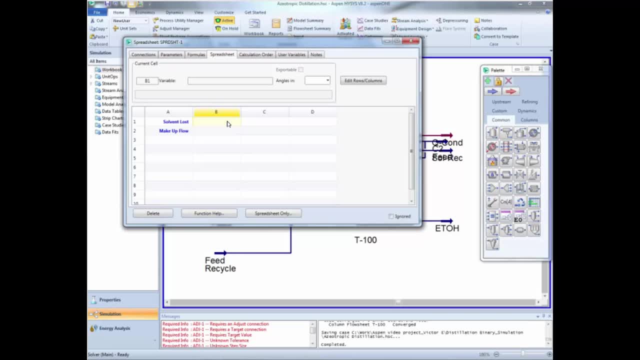 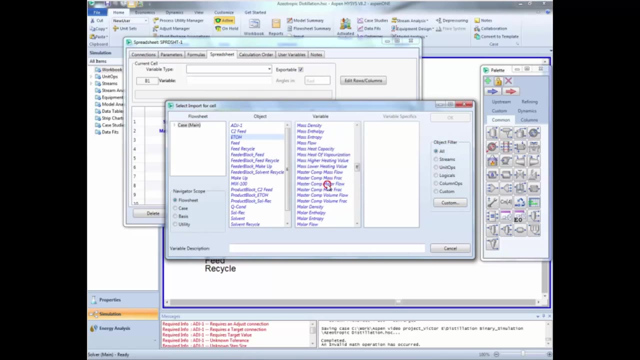 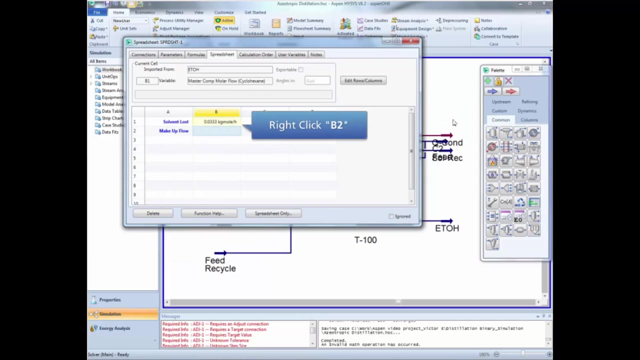 Now import the value of the cyclohexane molar flow in the ethanol stream in the cell B1, as shown in the video. In cell B2, import the molar flow of the makeup stream. Once you finish, close this window and click the save button. 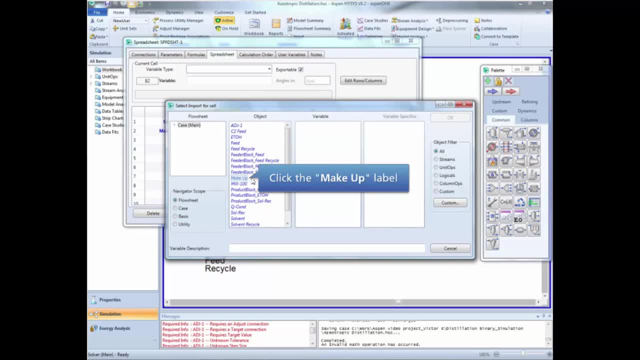 Now we are going to run the simulation of the distillation column. As you remember, at the beginning of the video, this warning message was known and these values were assumed in order to get a convert. simulation of the solvent, recycle and the makeup stream. 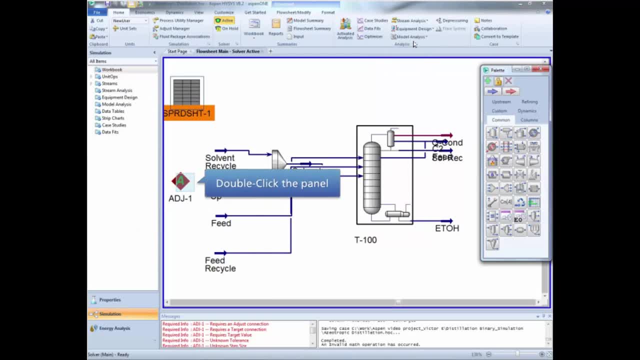 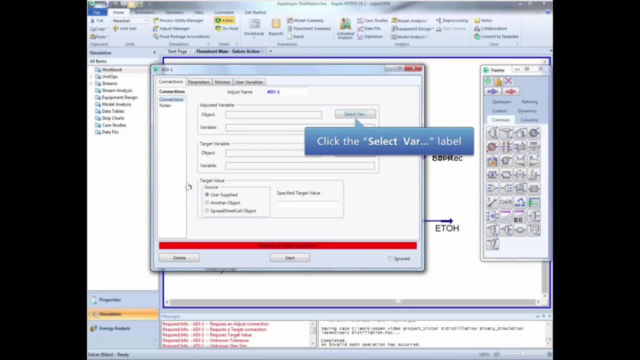 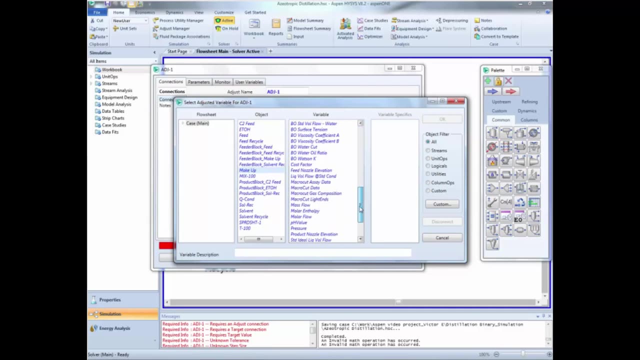 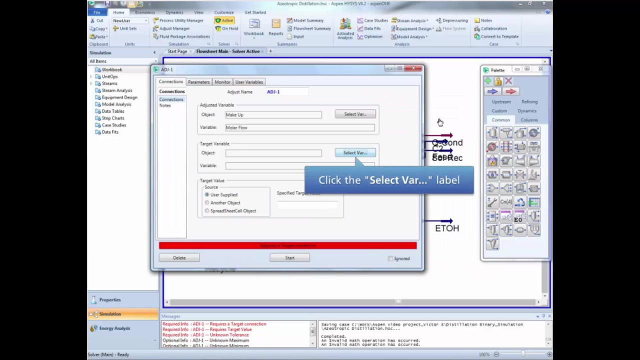 Now we are going to add a new value. Now open the adjustment block. Select the makeup stream, molar flow at the adjusted variable and the cyclohexane molar flow in the ethanol stream as the target variable. Now we are going to add a new value. 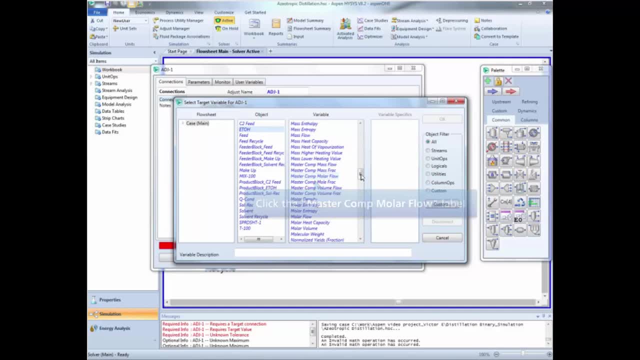 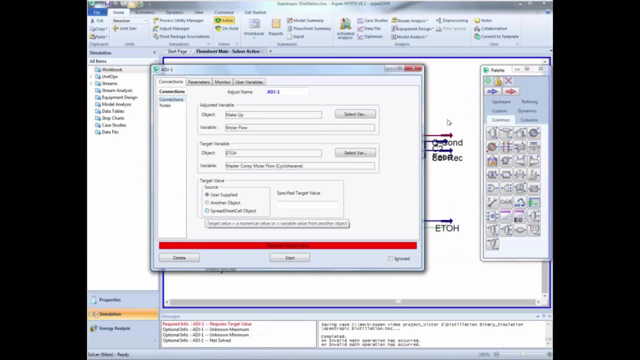 Now we are going to add a new value. We are going to add a new value. In the target value section, select the Source object to be a spreadsheet cell and, as matching value object, select the Cell B2.. Once you finish, go to the parameters tab. 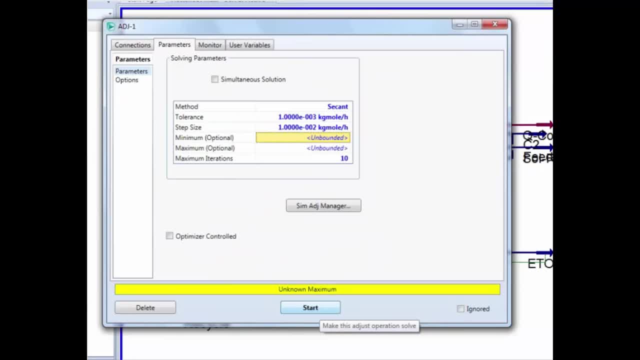 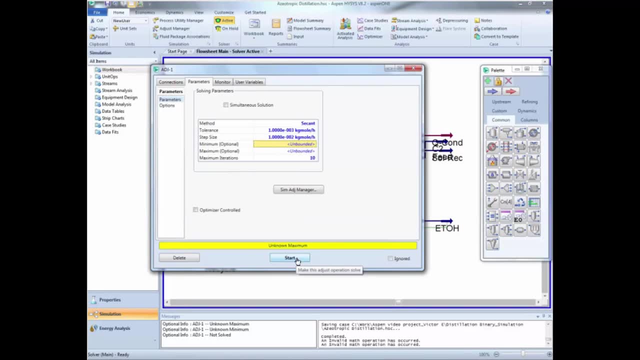 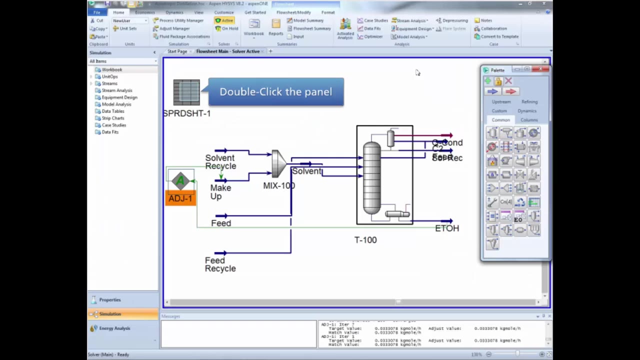 and change the tolerance and the step size as shown in the video. Click the start button and close this window to go back to the main flow sheet. Now open the spreadsheet again to see the result of what we did. As you can observe now, the makeup molar. 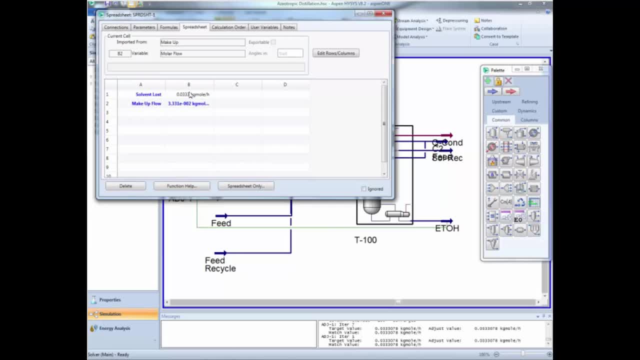 flow is the same as the saclohexane molar flow in the ethanol stream, which is the amount of solvent lost. But why do we need to do this? Remember that we mentioned that we want to minimize the waste of entrainer. For this reason we're 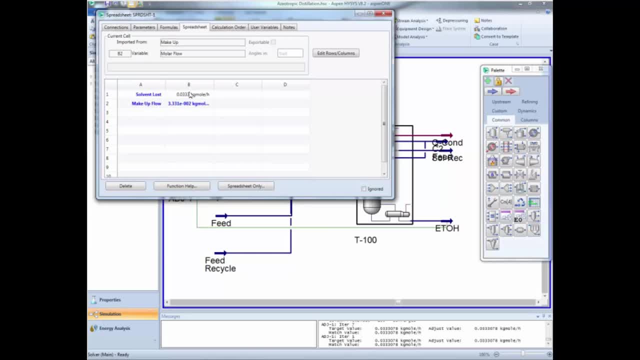 going to recycle back to the column the cyclohexane that leaves the column from the condenser. But if we don't do this, the simulation will never converge with a recycle because the entering molar flow of salgons of cyclohexane will 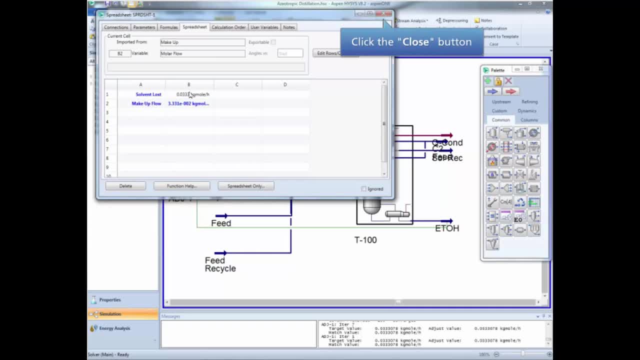 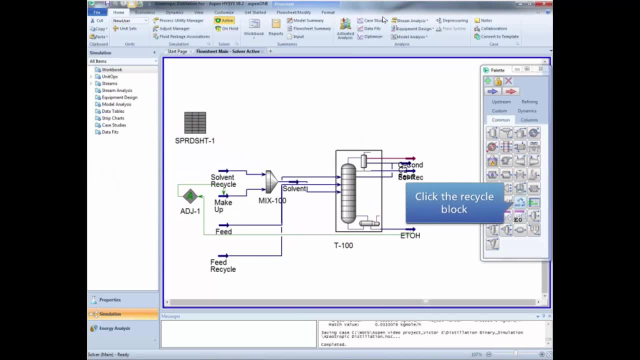 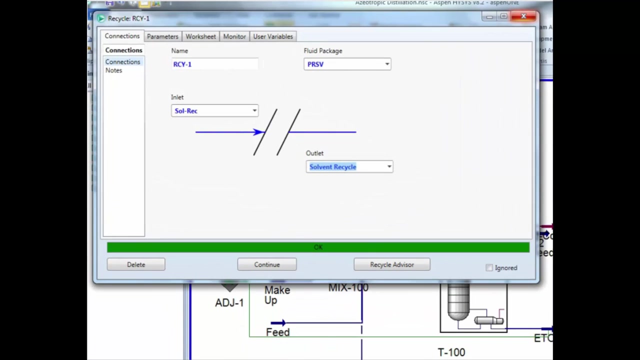 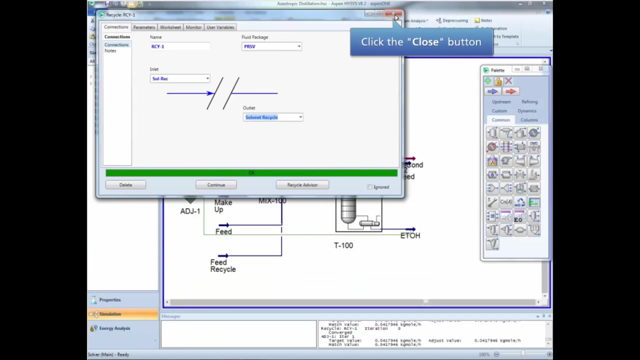 always be changing. Well, you can close this window now. Now we're going to add a recycle block. Double-click the item to open it. In this window, select the Solve Rake Stream as Inlet and the Solvent Recycle Stream as Outlet. You can close this window now. 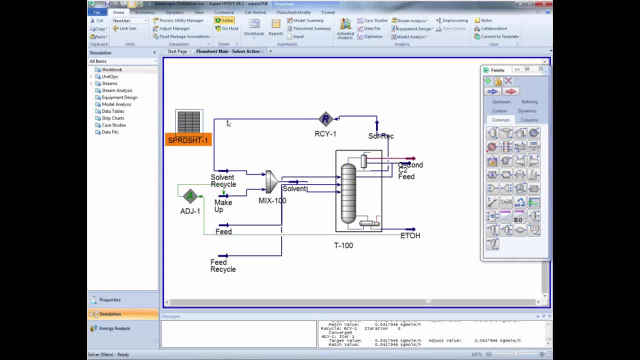 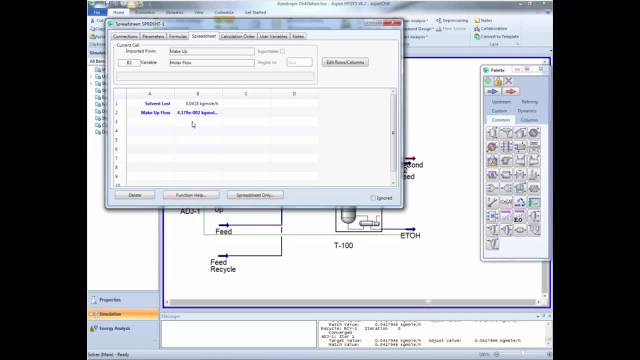 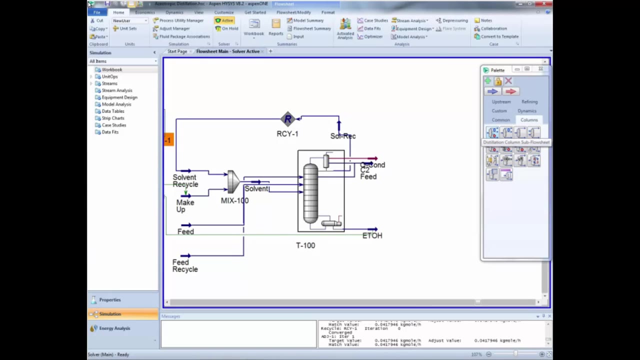 Now open the spreadsheet again to observe how the makeup molar flow is in agreement with the solvent lost in the ethanol stream. You can close this window now. In this section we're going to install a conventional distillation column to purify the water contained in the inorganic solution that leaves the 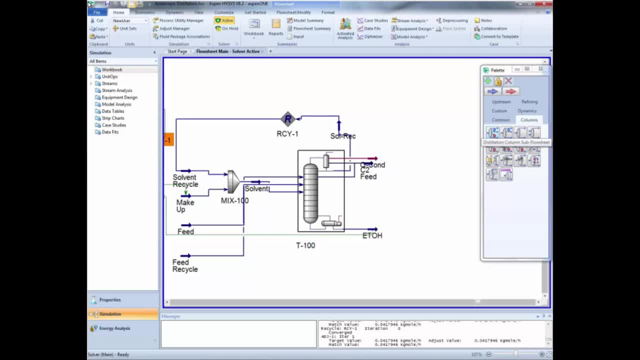 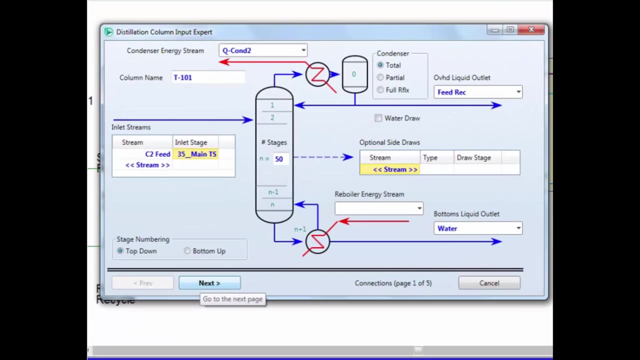 condenser. Then go to Columns tab in the palette and select the conventional distillation column item. On the first page of the columns of flowsheet write the following information: Number of stages: 50.. Inlet stream: C2 feet. Inlet stage 35.. Type of: 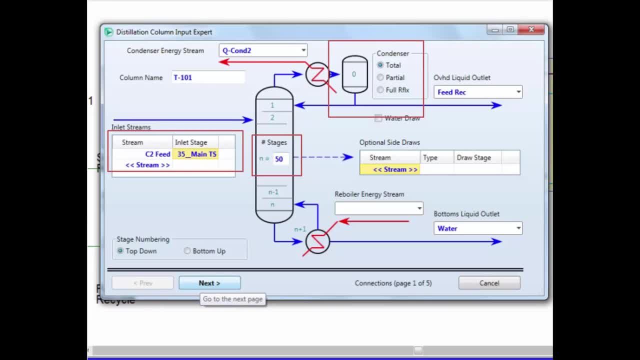 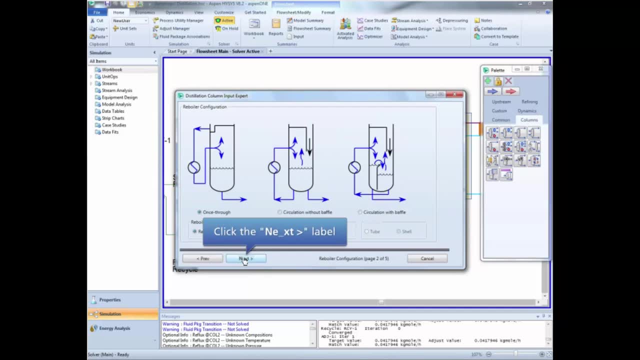 condenser total And write the names of the outlet and the energy streams as shown in the video. In the next page, leave the default re-boiler and click Next. Set the condenser and the re-boiler pressures to be 1 bar. This page asks for. 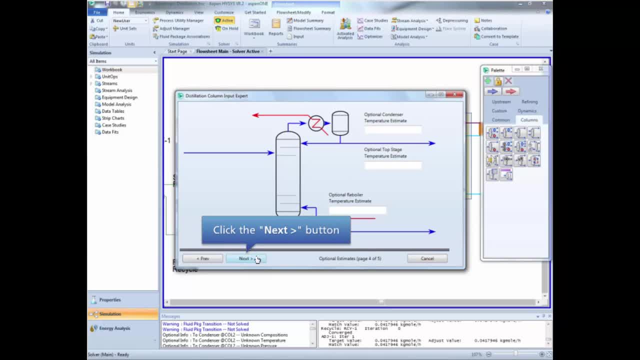 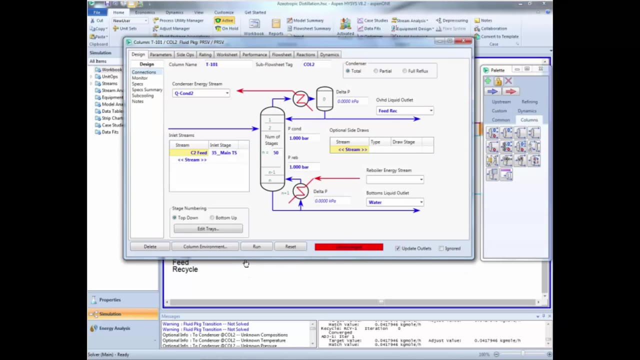 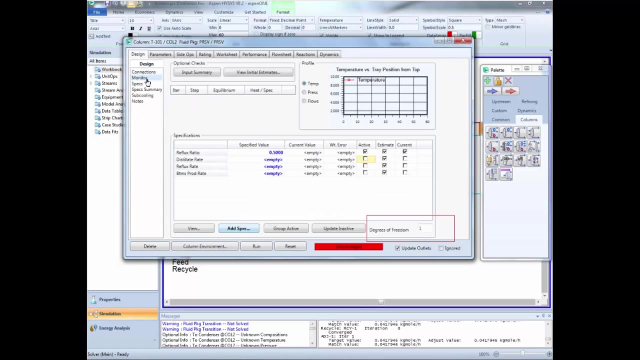 optional information. so we're going to leave it blank and click Next. Then we specify the reflux ratio to be 0.5 and then click Done. Now move to the monitors page to give the column specification and run the simulation. As you can observe, we still have one degree of freedom, so we're going. 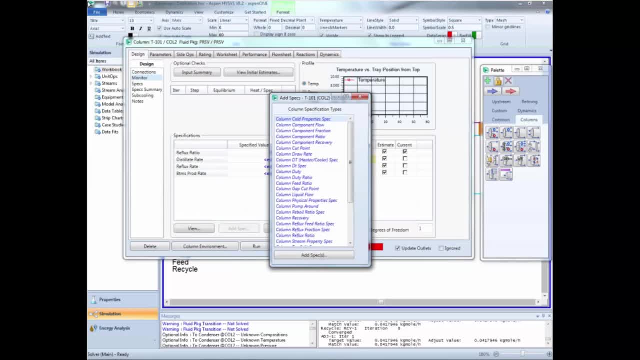 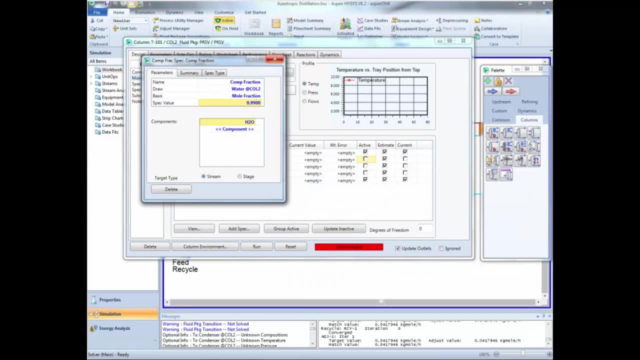 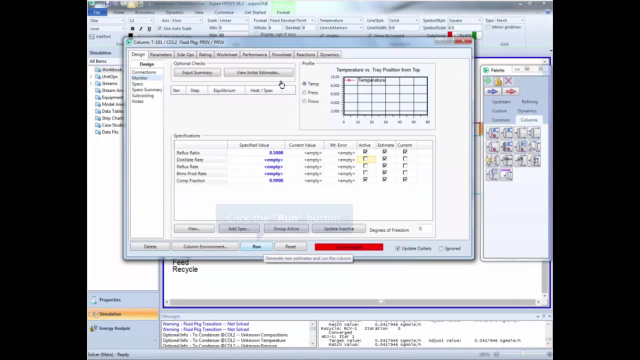 to add one specification. So we select a column, component, fraction specification, and then we write the specification, Click Run And now we have a converged simulation for the second column. You can close this window now. As mentioned at the beginning of the video, we want to minimize the